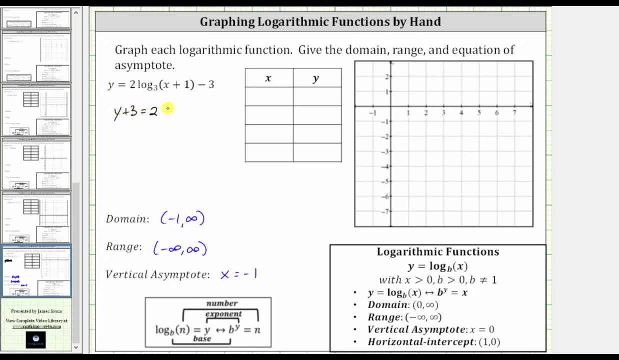 which gives us y plus three equals two times log base three of x plus one. And now we divide both sides by two, giving us the quantity y plus three divided by two is equal to log base three of the quantity x plus one. Now that we have the log by itself. 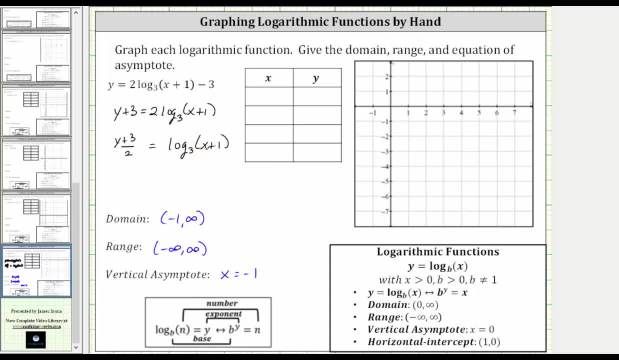 we now write the equivalent exponential equation using the definition below, which is: three raised to the power of the quantity. y plus three divided by two must equal x plus one. Again, the exponential equation is three raised to the power of y plus three divided by two. 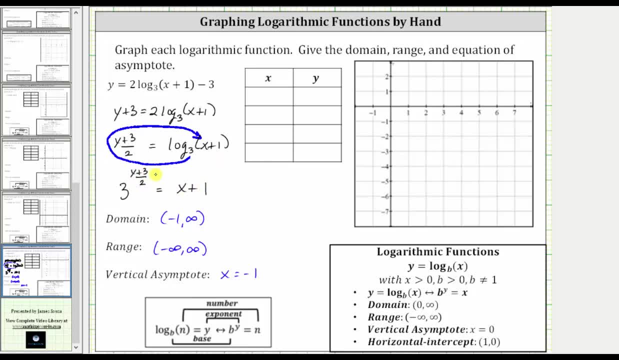 equals x plus one. Let's solve this for x, though before we complete the table. To solve for x we subtract one on both sides, which gives us the equation three raised to the power of y plus three divided by two minus one equals x. 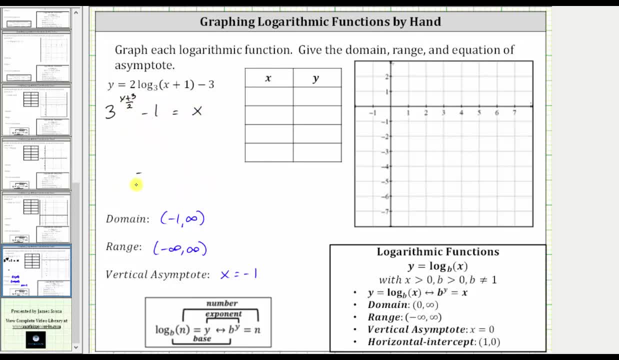 We will use this form of the exponential equation to complete the table. However, instead of selecting x and determining y, we will select y and determine x. Notice how, if y is equal to negative three, we would have a zero exponent here. So let's begin with: y equals negative three. 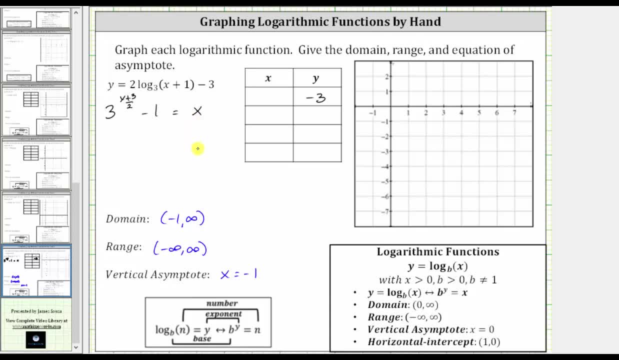 So again, when y is negative three, we have x equals. the exponent would be negative three plus three, which is zero. Zero divided by two is still zero. giving us three to the zero minus one. Well, three to the zero is one. 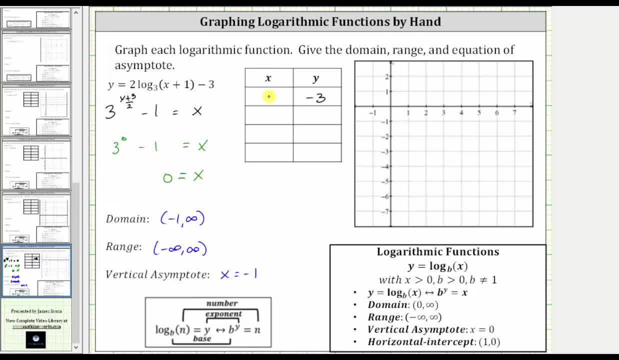 One minus one is zero. So we know the ordered pair: zero, comma negative three would be one point on the graph of the function. And now looking at the exponent, notice how we are dividing y plus three by two. So we do want y plus three to be even. 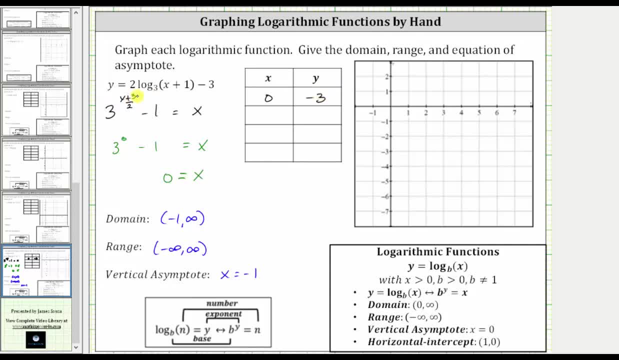 So if we increase negative three by two, the sum will still be even. Let's let y equal negative one. So when y is negative one, we have: x equals three. raised to the power of negative one plus three is two. Two divided by two is one.